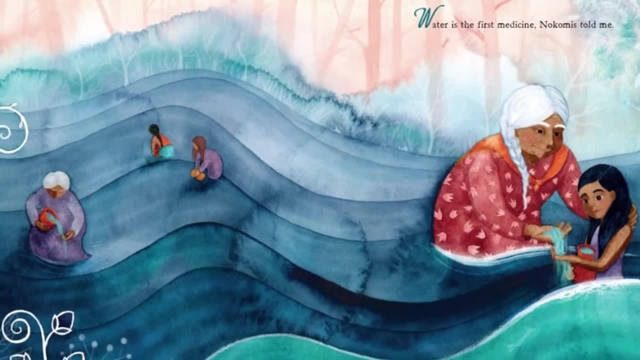 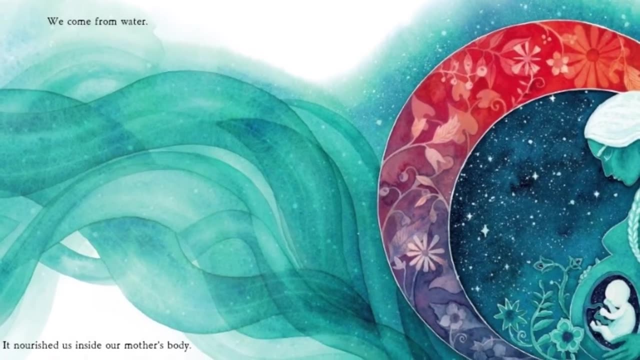 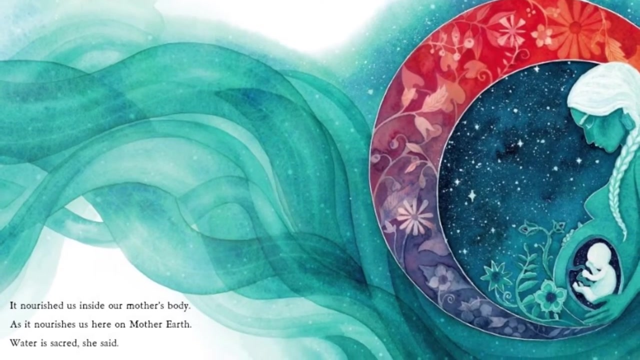 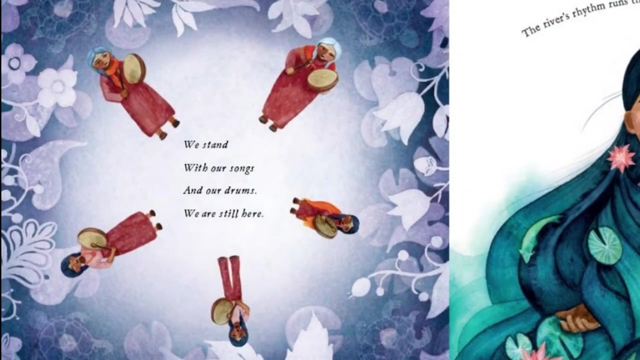 It's the first medicine Nukumis told me. We come from water. It nourished us inside our mother's body As it nourishes us here on Mother Earth. Water is sacred, she said. We stand with our songs and our drums. 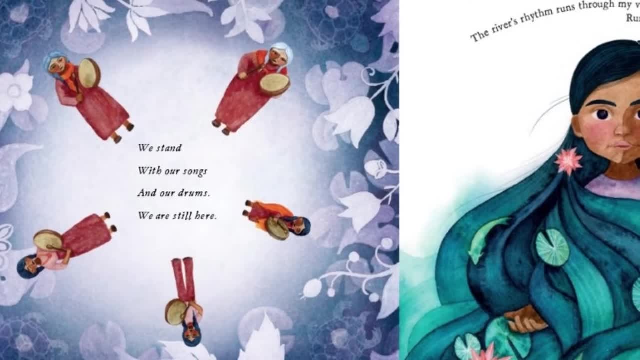 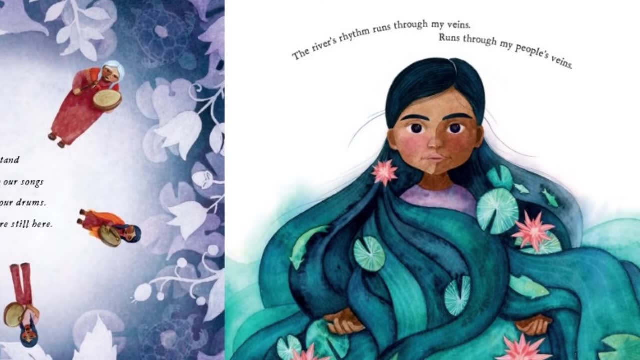 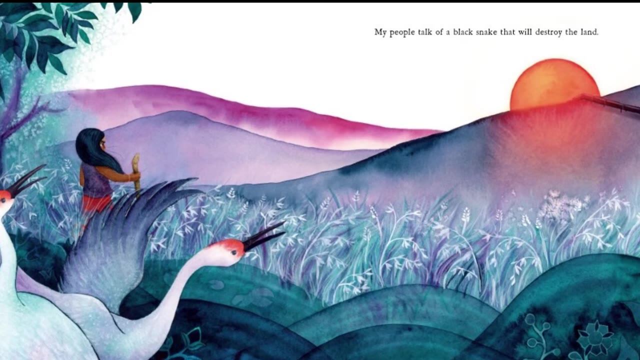 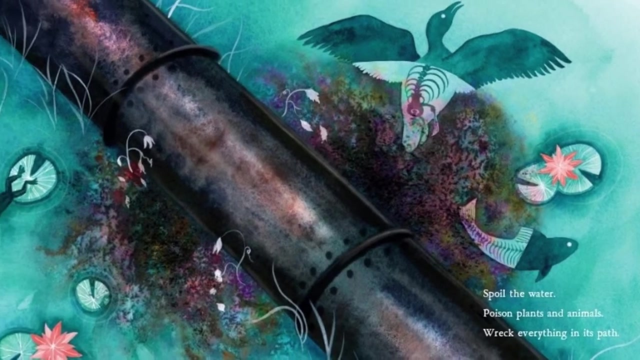 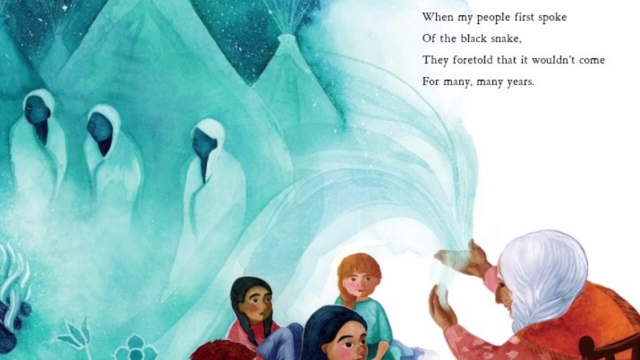 We are still here. The river's rhythm runs through my veins, runs through my people's veins. My people talk of a black snake that will destroy the land, Spoil the water, Poison plants and animals, wreck everything in its path. When my people first spoke, 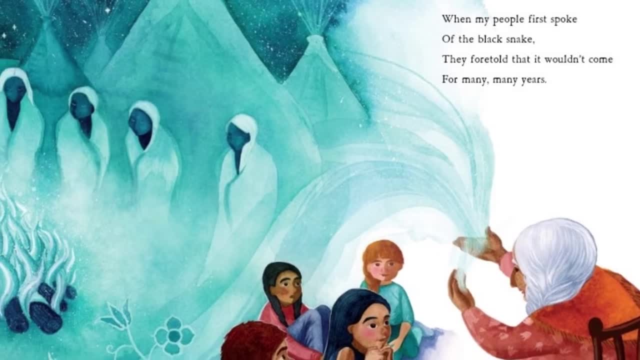 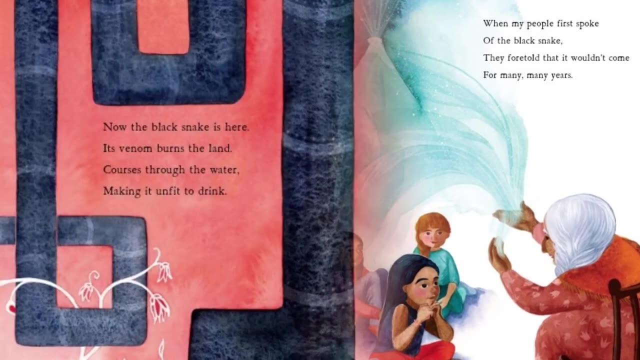 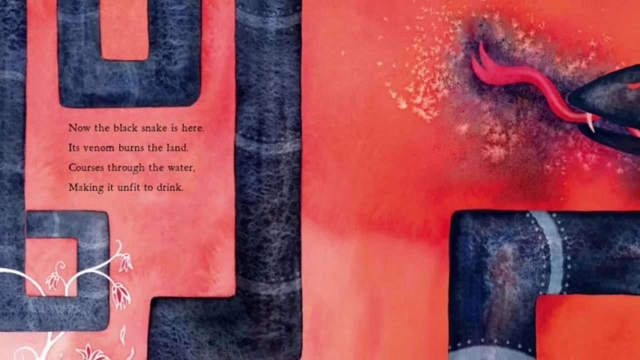 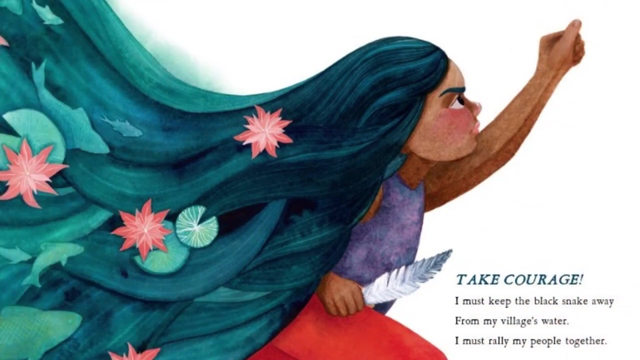 After a song Off the black snake, they foretold that it wouldn't come for many, many years. Now the black snake is here. Its venom burns the land, courses through the water, making it unfit to drink. Take courage. 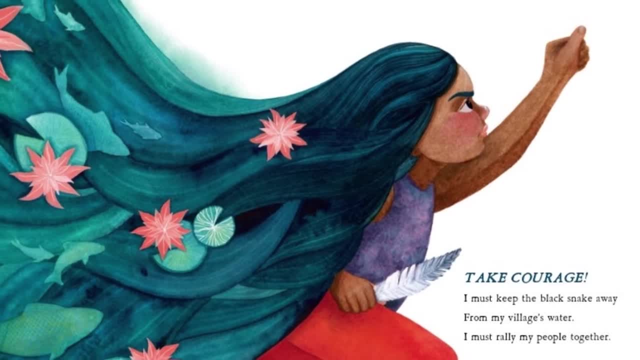 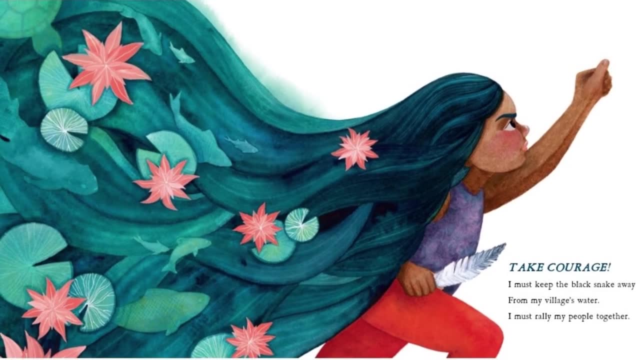 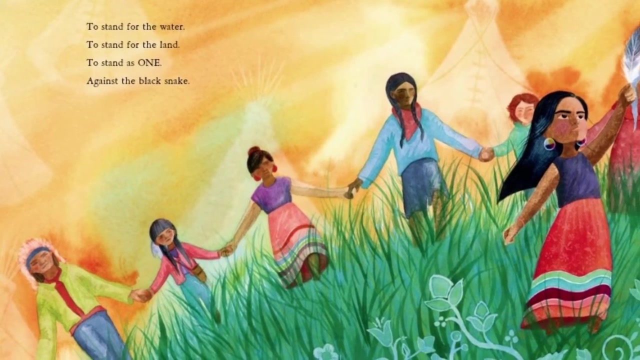 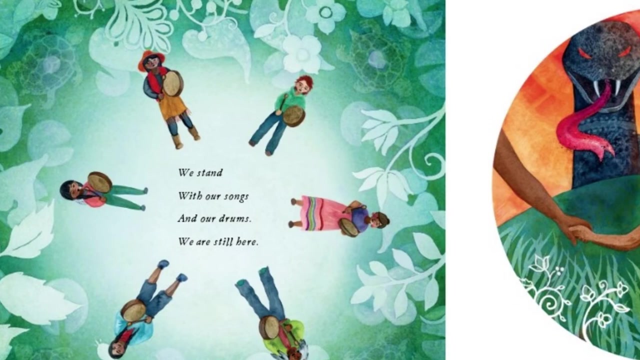 I must keep the black snake away from my village's water. I must rally my people together to stand for the water, to stand for the land, to stand as one against the black snake. We stand with our songs and our drums. We are still here. 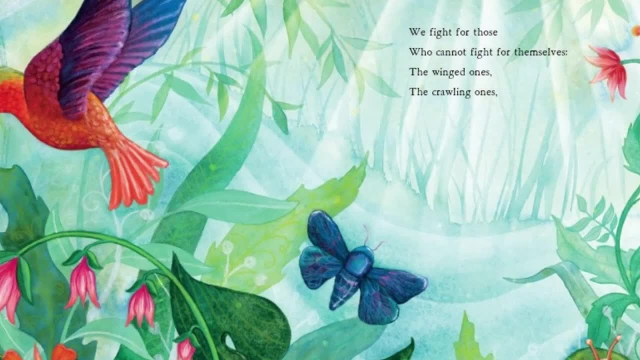 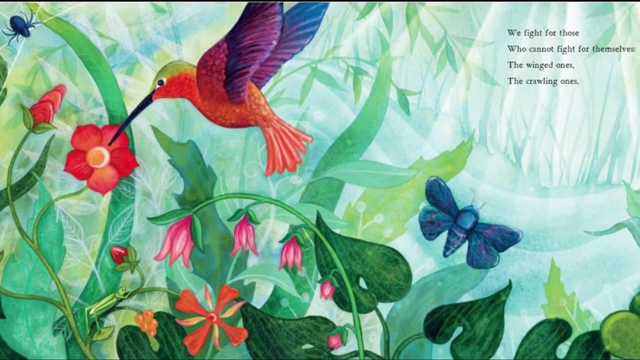 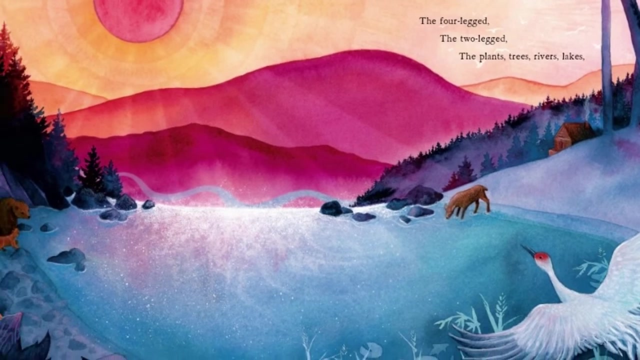 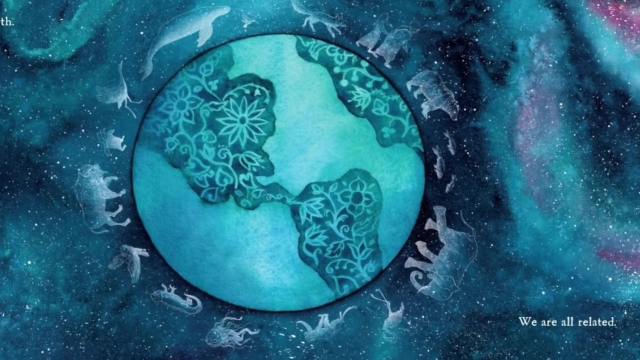 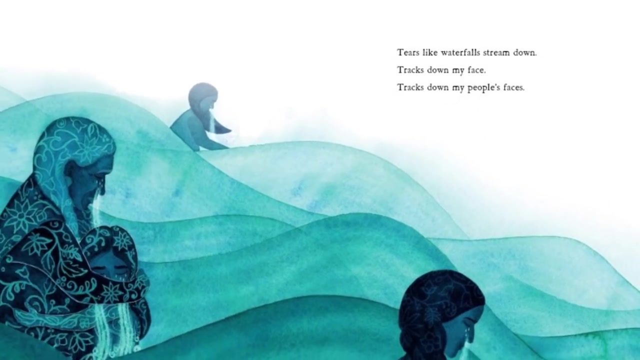 It will not be easy. We fight for those who cannot fight for themselves: The winged ones, the crawling ones, the four-legged, the two-legged, the plants, trees, rivers, lakes, the earth- We are all related. Tears, like waterfalls, stream down, tracks down my face, tracks down my people's faces. 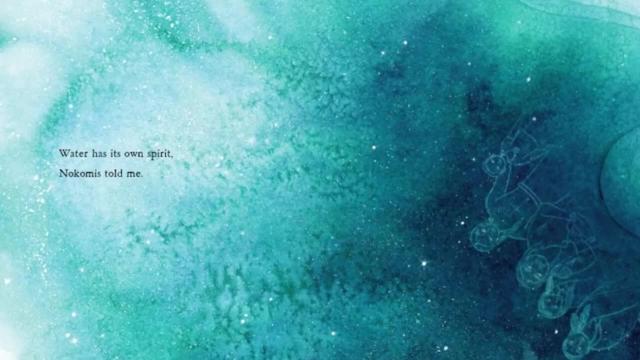 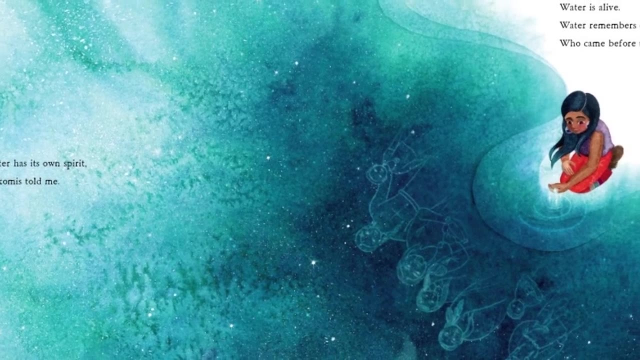 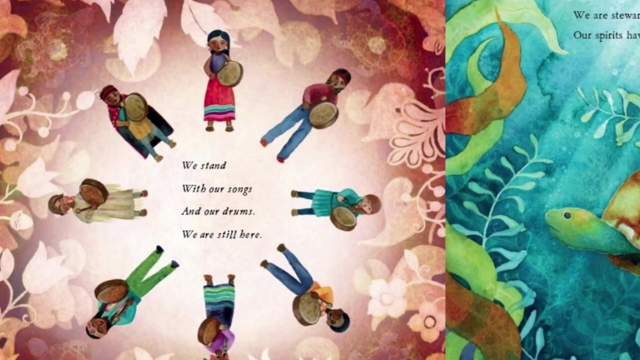 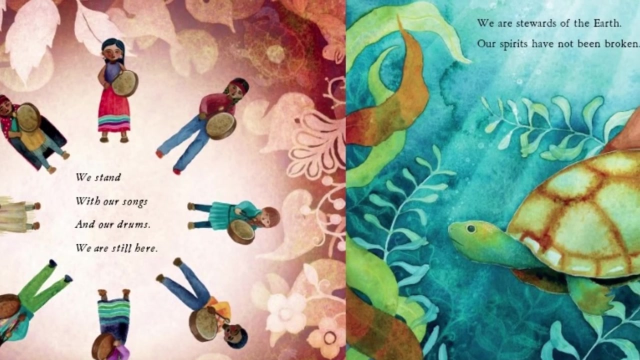 Water has its own spirit. Nukum has told me water is alive. Water remembers our ancestors who came before us. she said: We stand with our songs and our drums. We are still here. We are stewards of the earth. 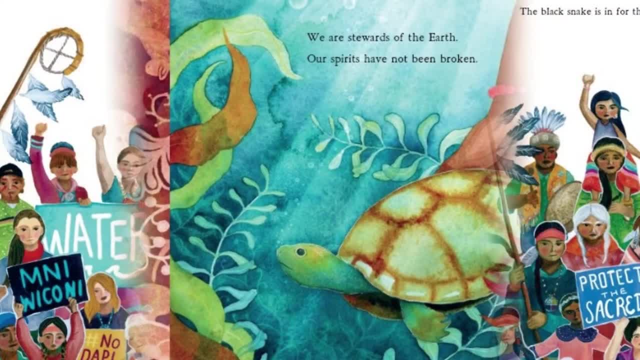 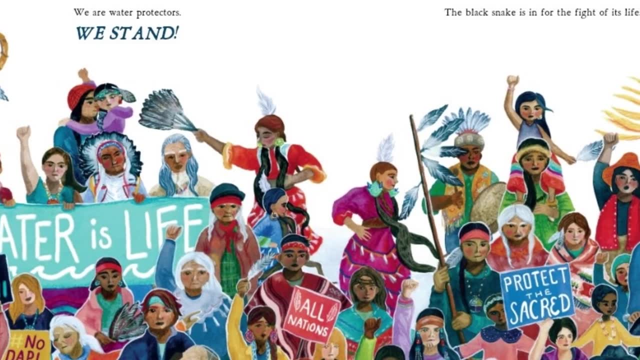 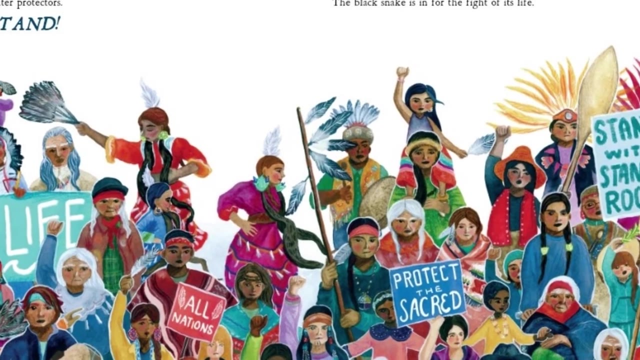 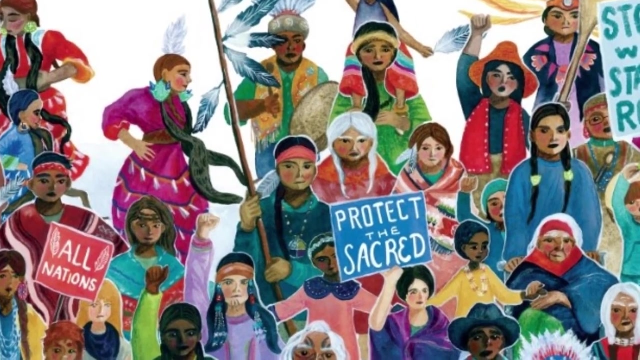 Our spirits have not been broken. We are water protectors. We stand. The black snake is in for the fight of its life, The end. I hope you guys really enjoyed this very important book that water is life. Save water and save mother nature. 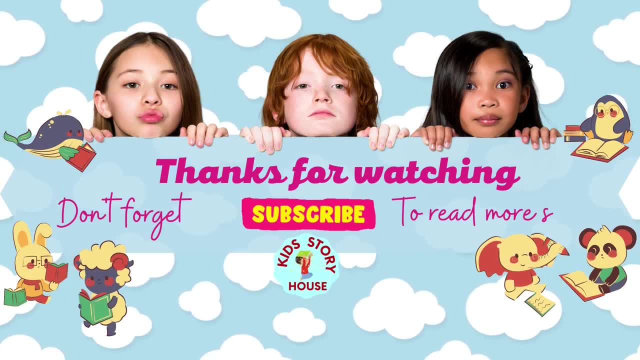 Bye-bye. Thanks for watching and don't forget to hit the subscribe button to read more stories. Bye-bye. 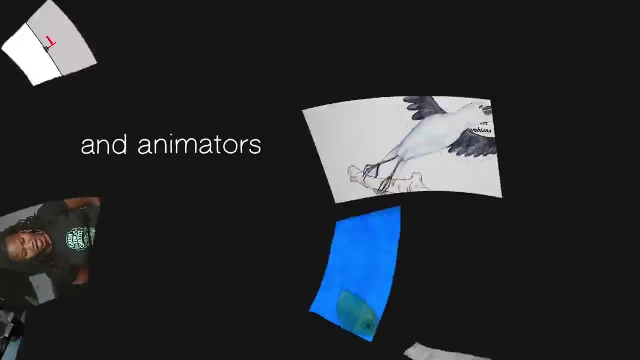 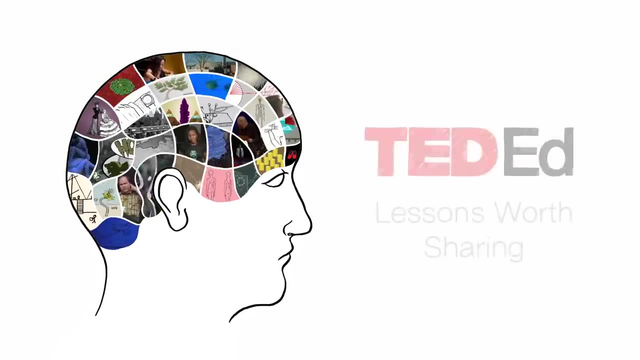 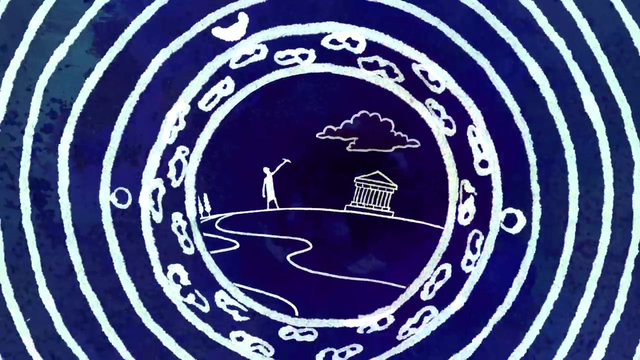 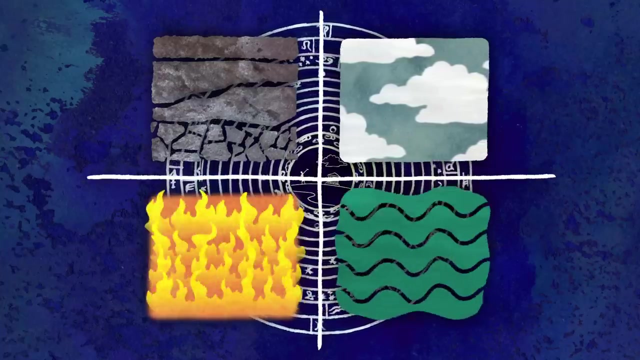 The ancient Greeks had a great idea. The universe is simple In their minds. all you needed to make it were four elements: earth, air, fire and water. As theories go, it's a beautiful one. It has simplicity and elegance. It says that by combining the four 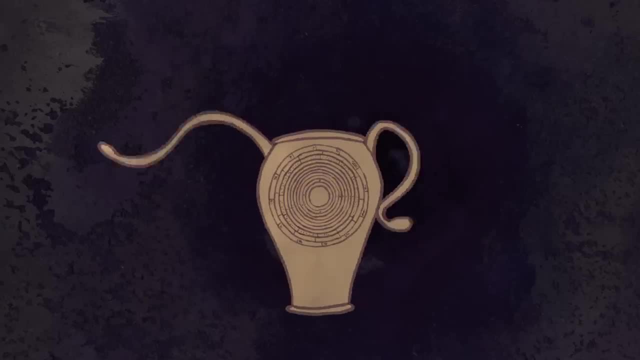 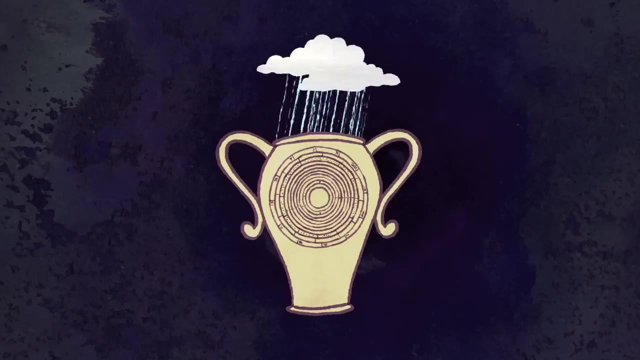 basic elements in different ways. you can produce all the wonderful diversity of the universe- Earth and fire, for example. give you things that are dry, Air and water, things that are wet, But as theories go, it had a problem. It didn't predict anything that could be measured. 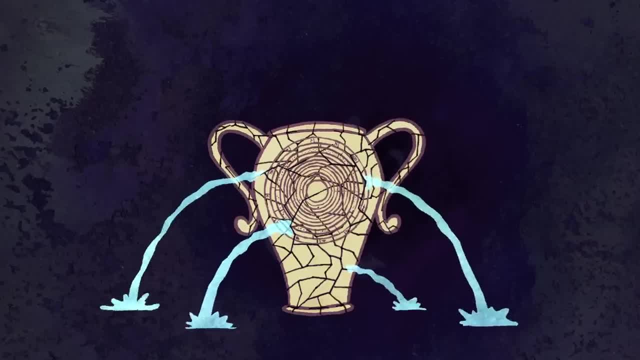 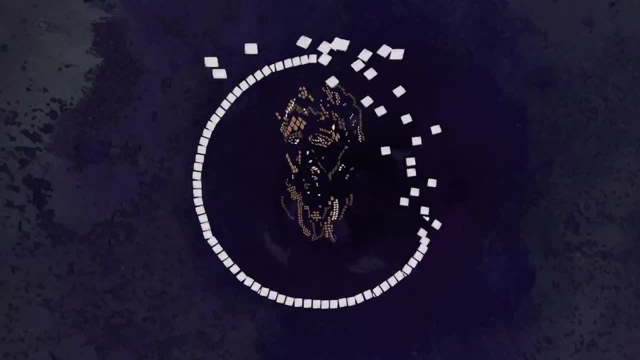 And measurement is the basis of experimental science. Worse still, the theory was wrong, But the Greeks were great scientists of the mind and in the 5th century BC, Leucippus of Miletus came up with one of the most enduring scientific ideas ever.